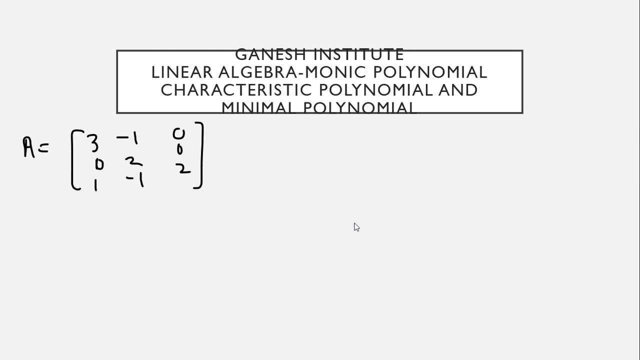 these three terms. okay, Terminologies. Let's take first up monic polynomial, right? So have you heard about monomial? It sounds something like that, right? But you have highest degree coefficient as 1 in monic polynomial. okay, So let's say: if I have x, 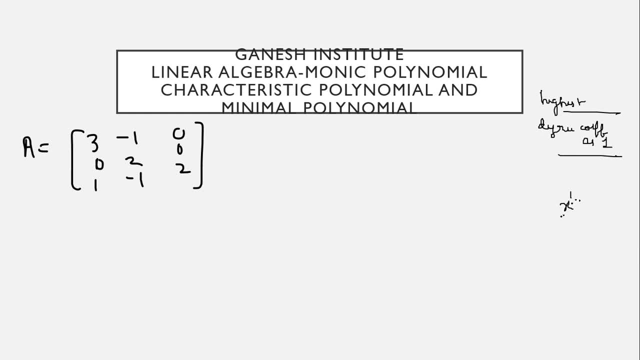 and its power is 1.. So this is monomial with linear degree. but its coefficient is also 1, so this is monic polynomial. But when we say characteristic polynomial, this is when we take up the example of matrix and find out a minus lambda i. This will give you characteristic. 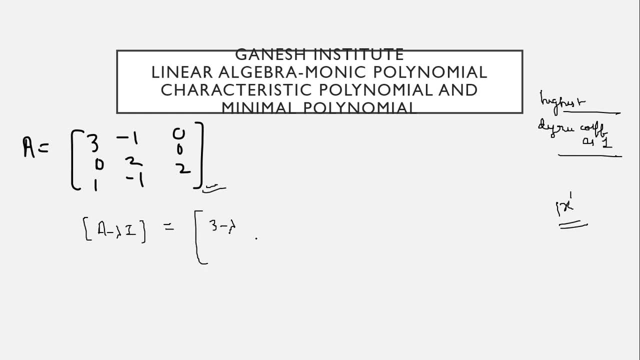 polynomial. So what it would be? 3 minus lambda, 2 minus lambda, 2 minus lambda. Rest. all other entries will be same. Do you know why? Because you know that identity matrix you are doing a minus lambda. i right, So i will be identity matrix of the same order as your matrix is. 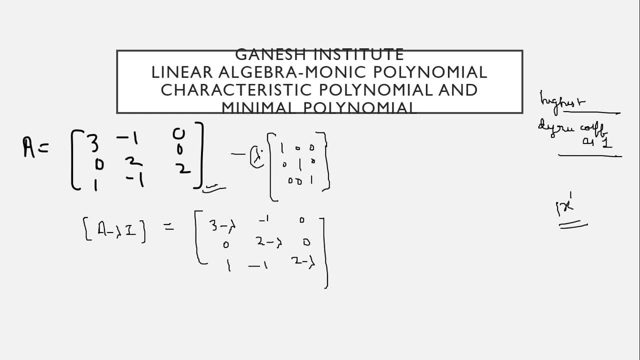 So you are multiplying it with lambda, So lambda will go and multiply it with these three. So if you subtract 3 minus lambda, you will get this Right. Rest: all elements will be as it is Now. this is the characteristic polynomial. 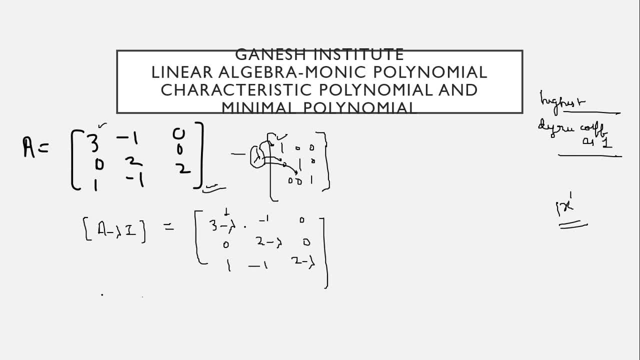 So if you have to find out the characteristic equation out of it, how would you do that? You will put a minus lambda i as 0. Correct, So you don't need to put it as 0. Just simply find out the determinant. Okay, So 3 minus lambda. 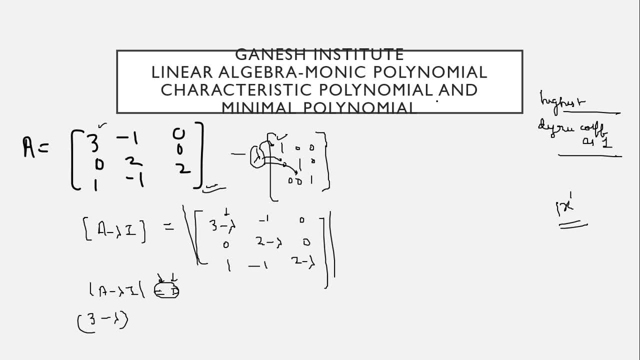 For equation you have to put it as 0. But at the moment we are trying to find out minimal polynomial out of it. So this is the difference between polynomial and equation. In equation you equate it with something that is maybe 0 or some number or some variable, But in polynomial 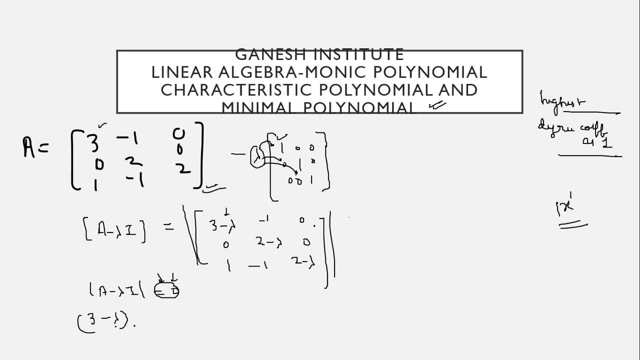 it is just expression. So 3 minus lambda will get multiplied with 2 minus lambda square and 0.. Right, So what I'm doing? I'm hiding this first row and first column where 3 minus lambda is lying. So, and take the determinant of the rest of the elements: 2 minus lambda square. 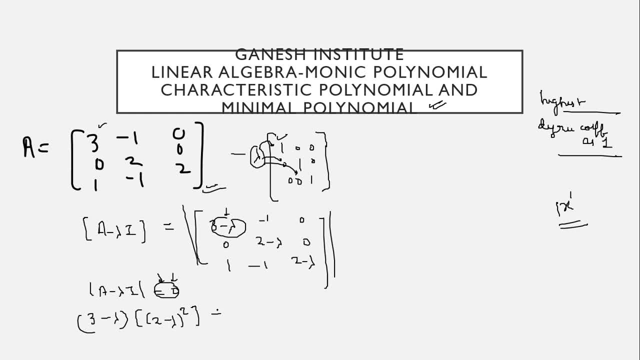 minus 0.. Then minus 1.. Minus is in the formula. Minus 1 makes it plus 1.. Hide this column and this row. It will give you 0, only Then 0. So only 3 minus lambda, 2 minus lambda- Whole square can be written as 2 minus lambda. Make it. 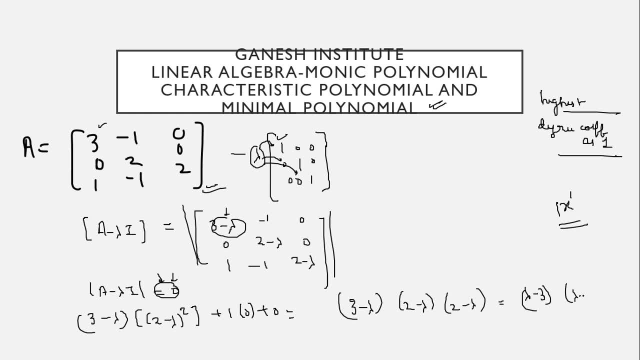 positive variable. Lambda minus 3.. Lambda minus 2.. So these two minus get cancelled, But for lambda minus 2, I'll be having minus here. So what are you seeing? Obviously, if I would have to find out eigenvalues, I would put these three as 0 and we'll get 3, 2 and 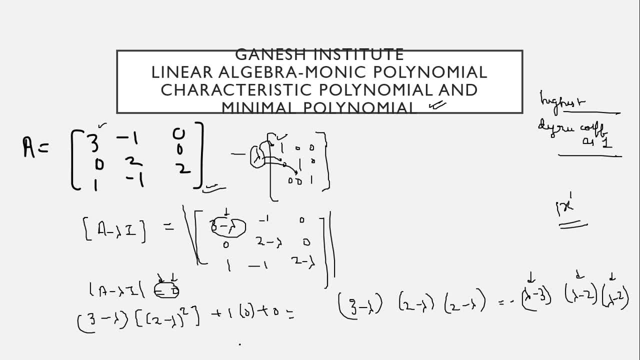 2 as eigenvalues. But here the question is: this is the characteristic polynomial. We've found it, But how can we calculate minimal polynomial out of it? So remember, when we have to find out minimal polynomial, then it's power, It will be extracted from characteristic polynomial, only. That's. 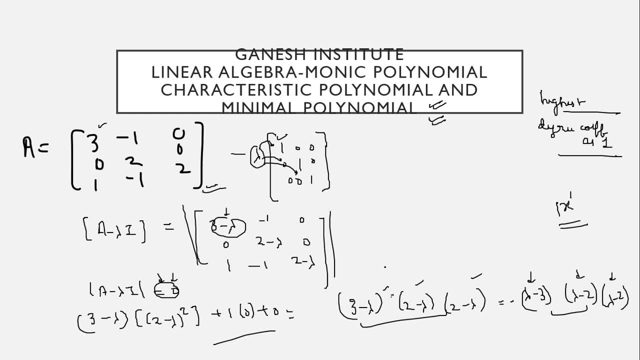 why it's power. The variable will be having power lesser or equal than characteristic polynomial. Okay, Okay, So it might be the case that the polynomial which can be of smaller size from it, it can be lambda minus 3, lambda minus 2.. Because then? because you can see, this is the cubic. 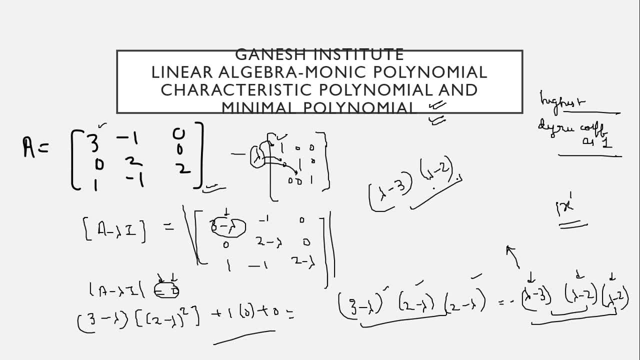 polynomial Correct, So it can be either cubic or quadratic or linear, but not more than that, Getting my point. So lambda minus 3, lambda minus 2 is one case, Or lambda minus 3, lambda minus 2.. Okay, 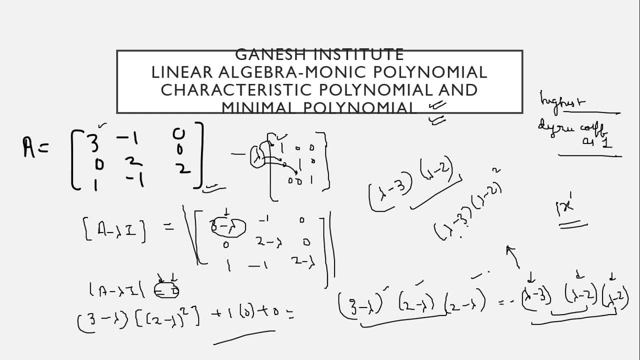 The whole square is one case. Now, if you take lambda minus 3, lambda minus 2, this one, and if you multiply it, what will you get? Lambda square minus 5, lambda plus 3 to the 6. Right. 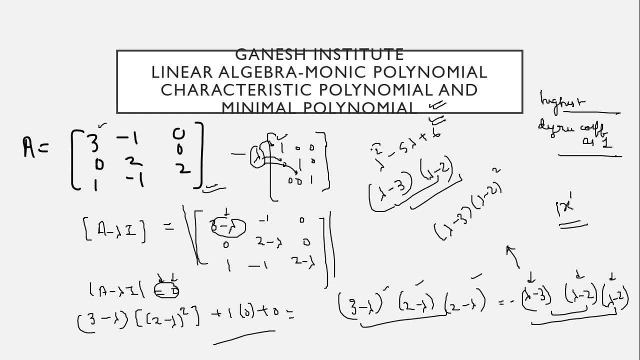 And this is something: when you will get the least degree of lambda, Here also your degree will be equal to the main polynomial characteristic polynomial. But as soon as you get the least degree of lambda, as soon as you get the degree lesser than the characteristic polynomial, 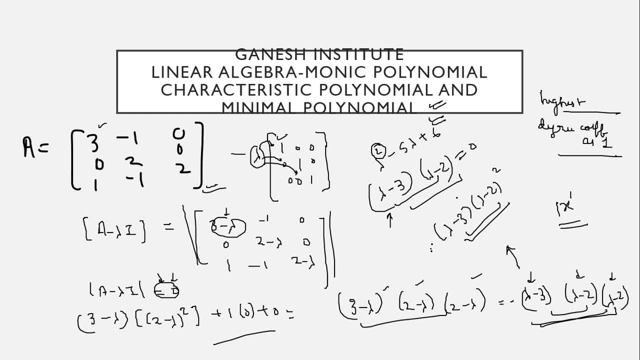 and it satisfies the values, then this can be considered as minimal polynomial. So minimal polynomial is lambda minus 3 into lambda minus 2.. Hope you understood it And if so, then don't forget to like, share and subscribe my channel Till my next video, take care. of yourself. Bye, bye. 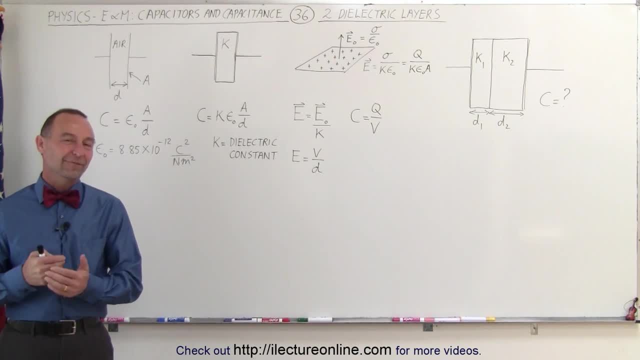 Welcome to Electron Line. There are some viewers that asked if I had videos on capacitors that had multi-layer dielectrics. It turned out I do kind of, but not really So here's some very straightforward examples of how to calculate the capacitance of a capacitor that has two. 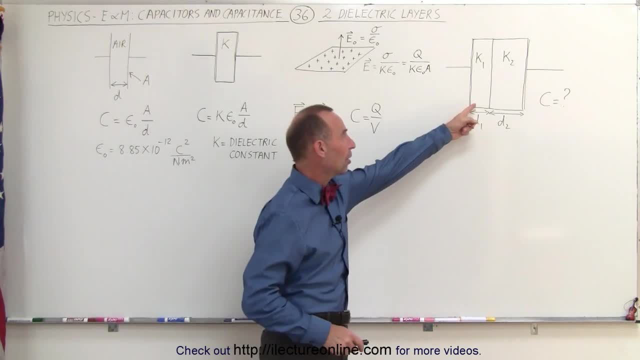 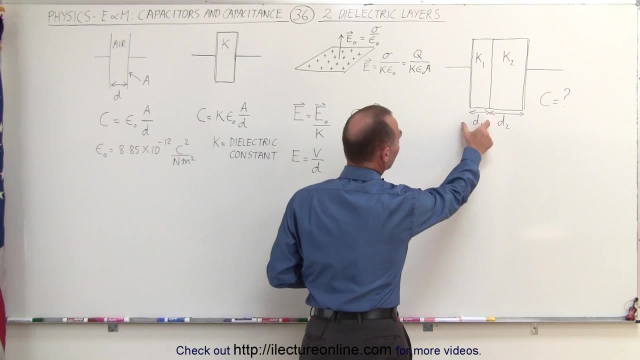 dielectric layers in it. So here's the picture of what we're trying to solve. We're trying to find the capacitance of this particular capacitor. Notice that the thickness of each dielectric can be any thickness, so call it d1 and d2, can be any values and the dielectric constant k1 and k2 can. 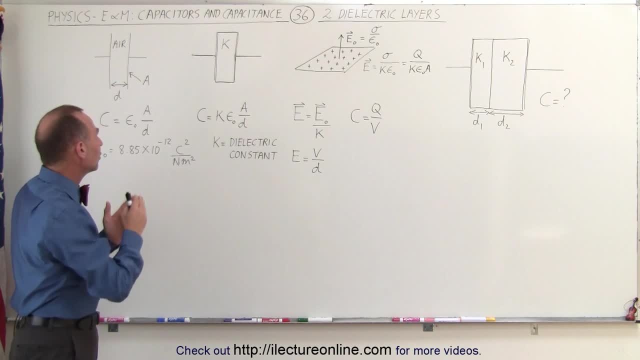 be any value as well. So how do we do that? Let's go back to the beginning, and here's a simple capacitor with air between the plates. The capacitance for a physical capacitor is equal to epsilon sub naught times the area of the plates divided by the distance between the plates, where 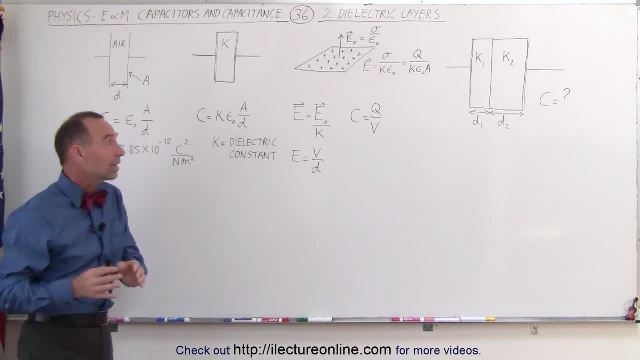 epsilon sub naught is given right here. If there's a dielectric in there, then you have to multiply that capacitance times the area of the plates divided by the distance between the plates where epsilon sub naught is given right here. If there's a dielectric in there, then you have to multiply that capacitance. 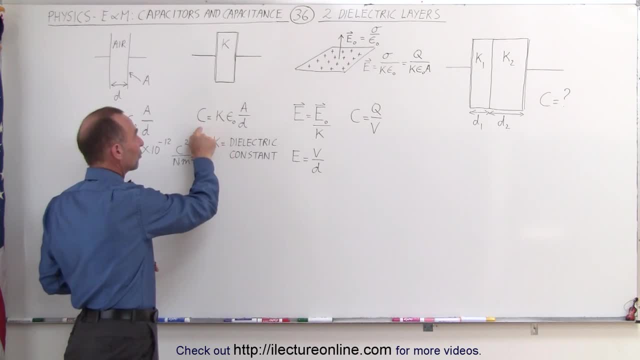 times the dielectric constant and you can see that a capacitor with dielectric has a greater capacitance than a capacitor without the dielectric. another few things that we need to know. first of all, that the electric field between the capacitor plates will be diminished by the dielectric.